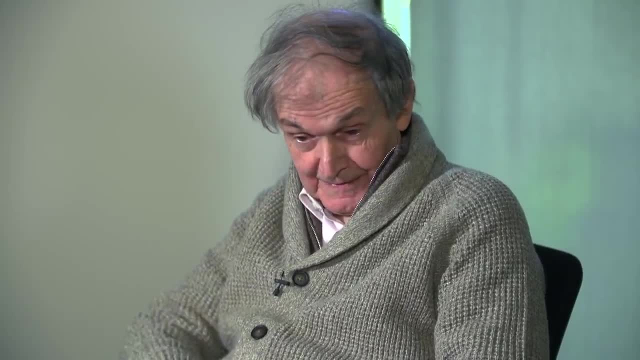 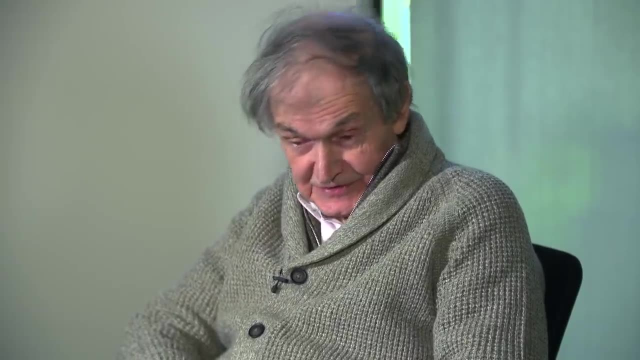 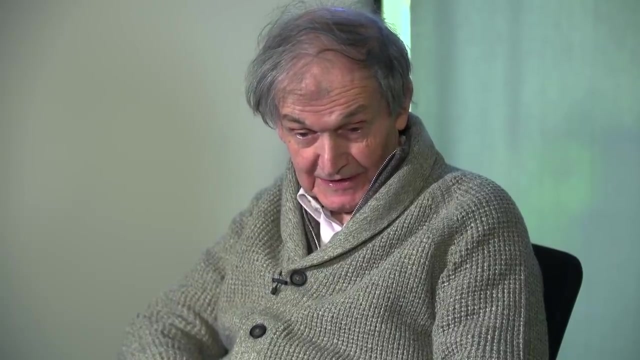 governed by this wonderful equation due to Erwin Schrodinger. The trouble is that it doesn't. That's to say, the way physicists usually use the Schrodinger equation is to work out certain probabilities of what an observation on the system would tell you. So what you? 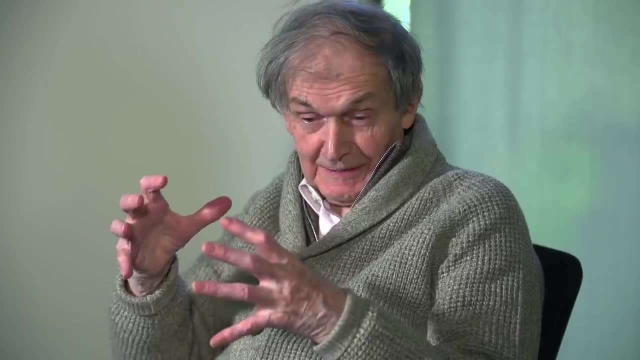 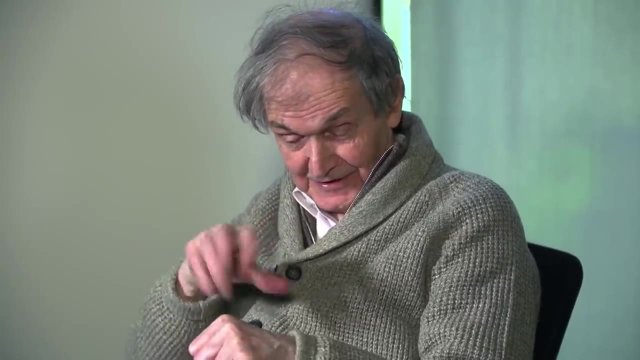 have to do is you wheel out of the cupboard a measuring device And this measuring device, you set it on the system, which is evolving according to the Schrodinger equation, and it measures it, And the process of measurement does not follow the Schrodinger equation. 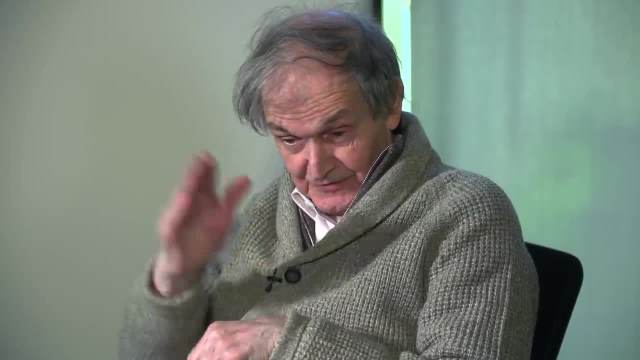 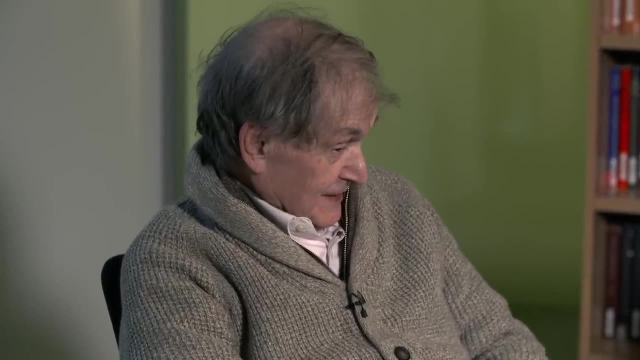 It gives you a probabilistic answer: this or this or this. That's another outside-the-system problem. Well, it's certainly outside the Schrodinger equation, Right, right, right, And Schrodinger was terribly worried about this. I mean, he produced his cat in a box. 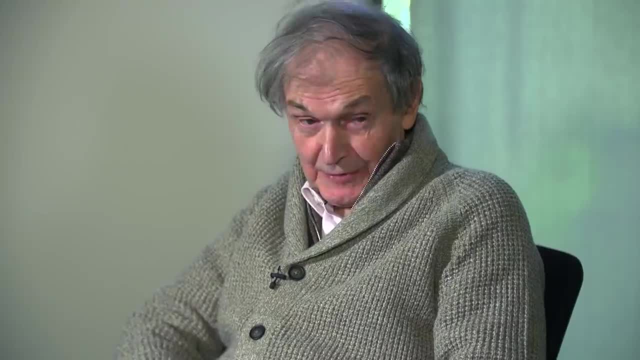 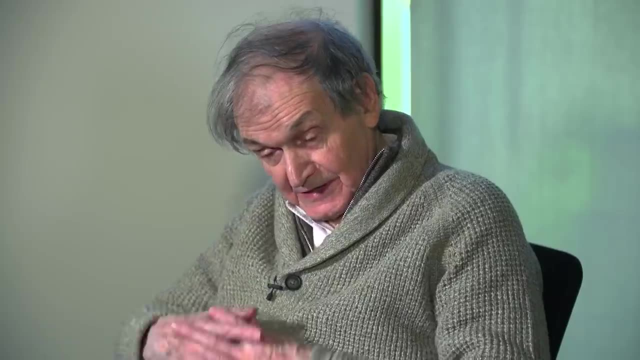 and all sorts of things. You see, he clearly realized there was a problem, as did Einstein. There's no question about that. Some others didn't. Well, they took a different view. They said: look, we don't understand the theory well enough, And that's more that we're saying. Where Schrodinger was not saying that, He was saying: well, you don't understand the theory well enough, And that's more that we're saying. Where Schrodinger was not saying that, He was saying: well, you don't understand the theory well enough, And that's more that we're saying. 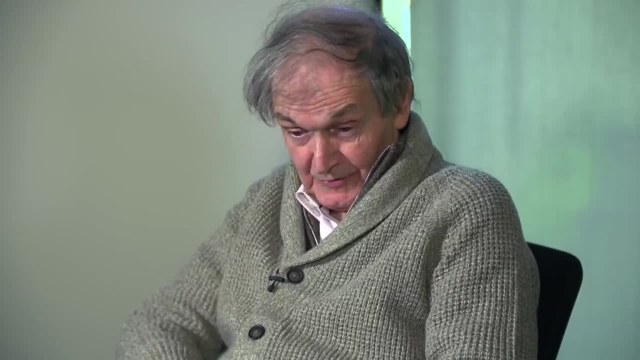 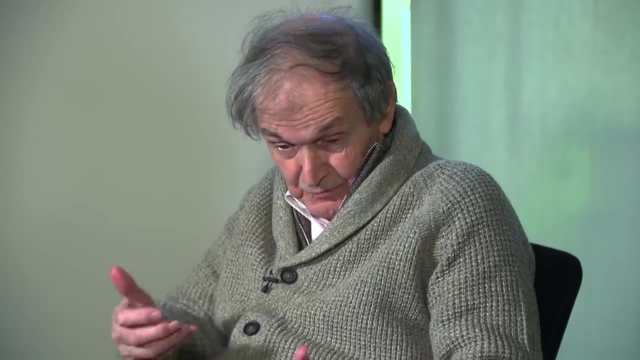 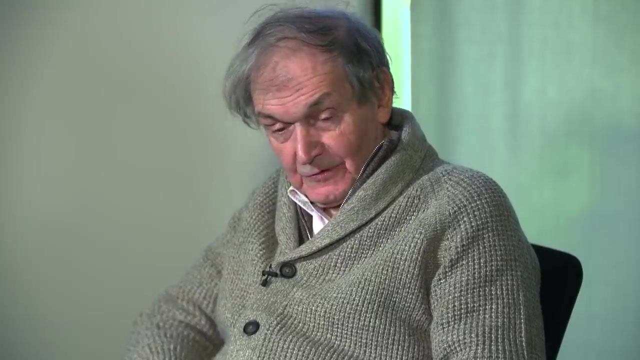 We understand it well enough to see that that's not the way the world operates. When you make a measurement on a system, it does not follow the Schrodinger equation, And that's what people understand about quantum mechanics, But it's a sort of vague set of rules about 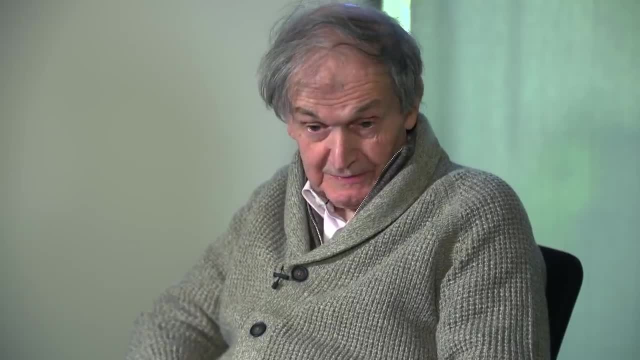 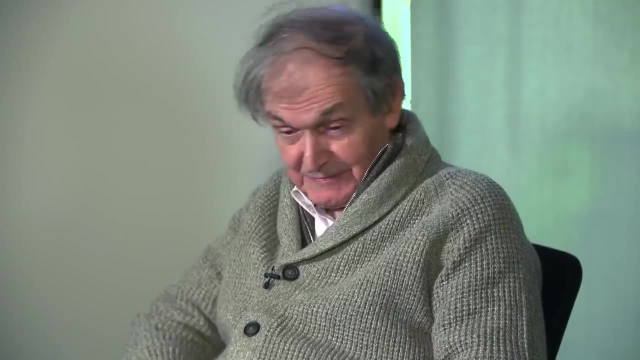 it doesn't tell you what constitutes a measurement. Right, That's the trouble. Right, Yeah, that's a big trouble. actually, That's the big trouble, Yeah, yeah. They say, if you do a measurement then it just becomes a probability. for what? 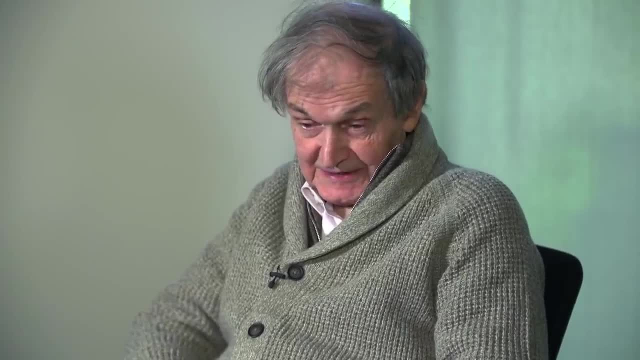 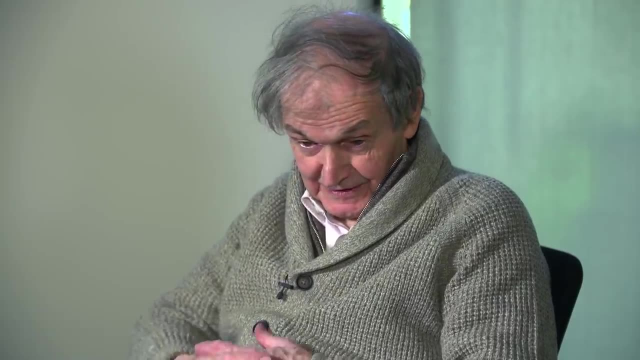 this or that or the other, But it doesn't say what kind of a device makes a measurement. Now there's one school of thought which has been going on from way back to the early days of quantum mechanics. Wigner, in particular, promoted this point of view: that it's a conscious. 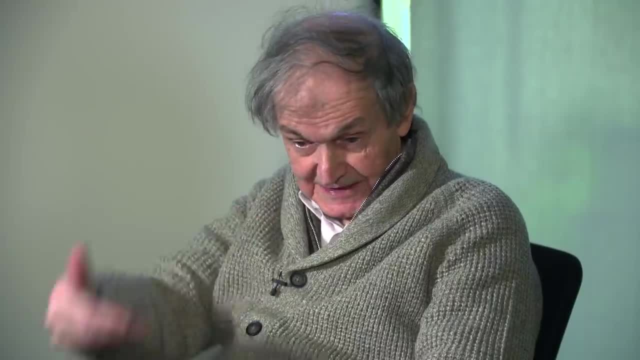 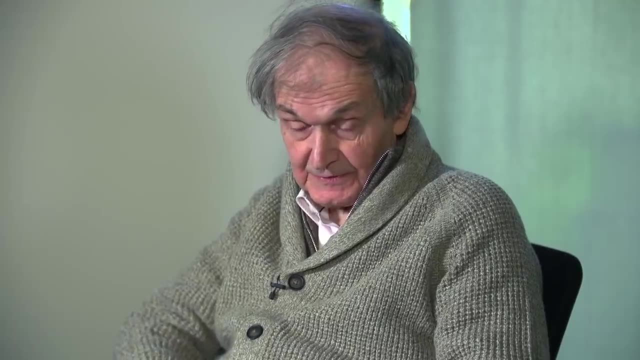 being observing the system And that makes the. That's what Wheeler believed. I believe Wheeler might have believed. quite a lot of people believe that. I think von Neumann had a similar sort of view. I'm not quite so sure about his view, But certainly Wigner. 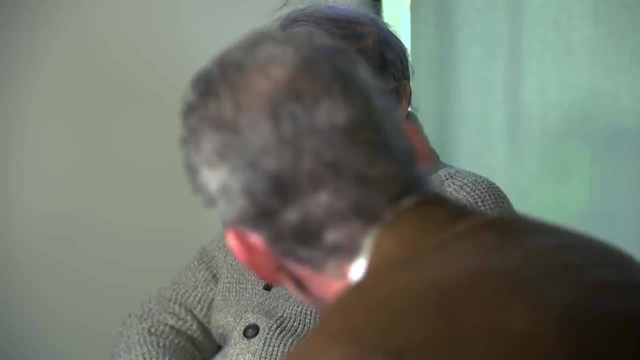 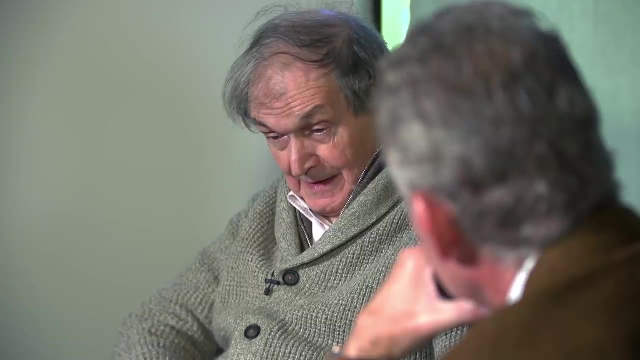 And I talked to Wigner about it. Yeah, I got the feeling from Wigner he wasn't quite as dogmatic He was made out to be on this issue. He just thought this was a possibility, I think. But anyway, that's people often. 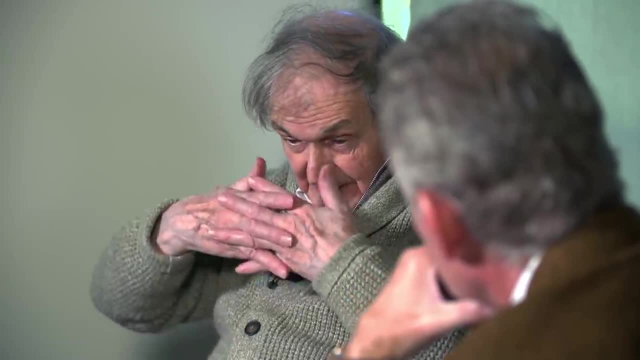 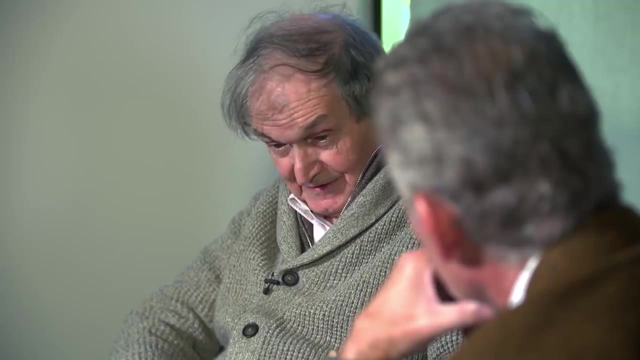 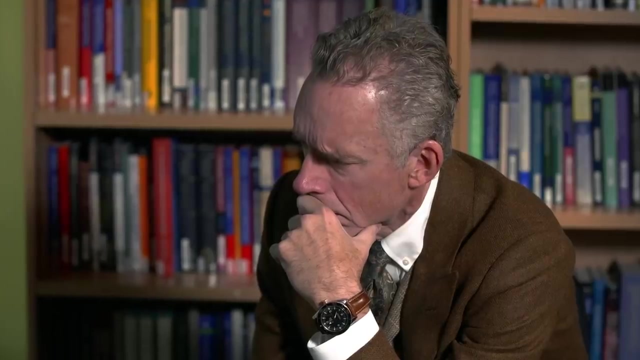 refer to it as the Wigner view that it's a conscious being who makes the measurement. That's not my view. My view is that it's almost the opposite of that view, that there is an objective physical process which deviates from the Schrodinger equation, in which the state does collapse. 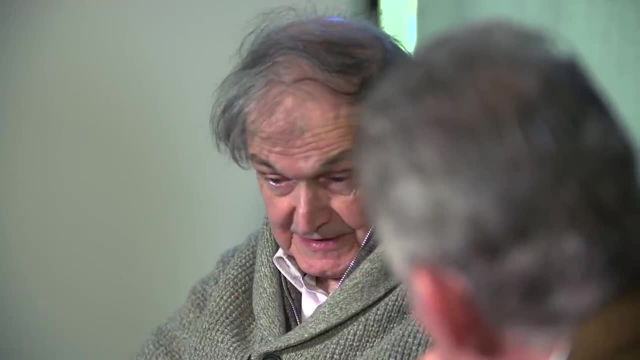 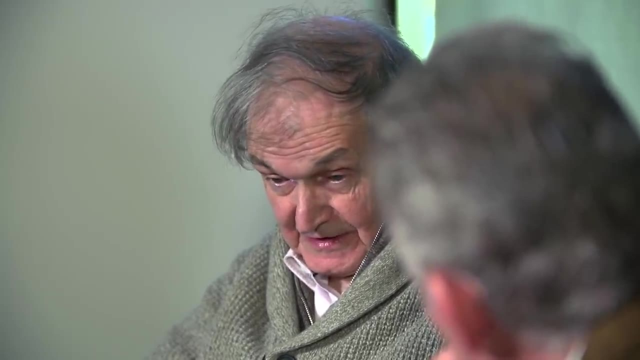 so that it becomes one or the other or the other with certain probabilities, And that this has to do with when gravity is brought into the picture, And there's reasons for believing this. I don't want to go into that, But there is reason for seeing. 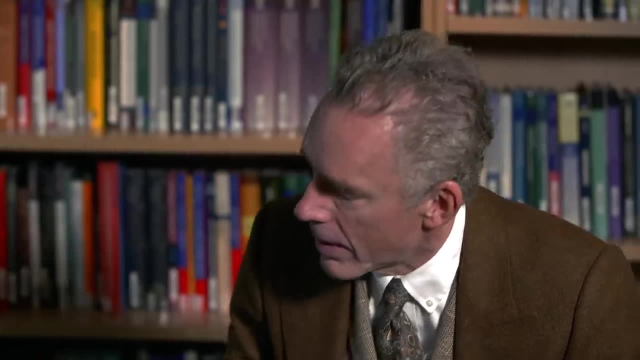 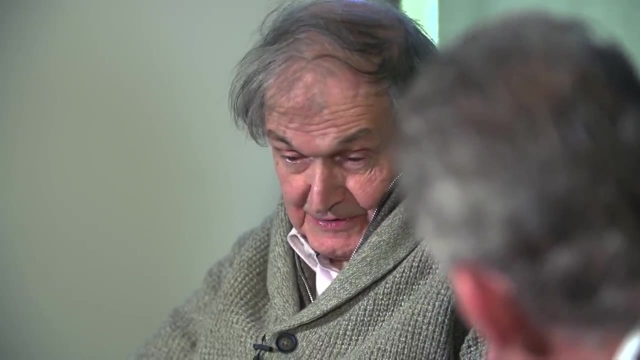 I'd like you to go into it if you would be willing to, Because, I mean, I'm very Well. it's a very clear mathematical calculation. There's not a question about it. It's a question of what you do with it. you see, And what. 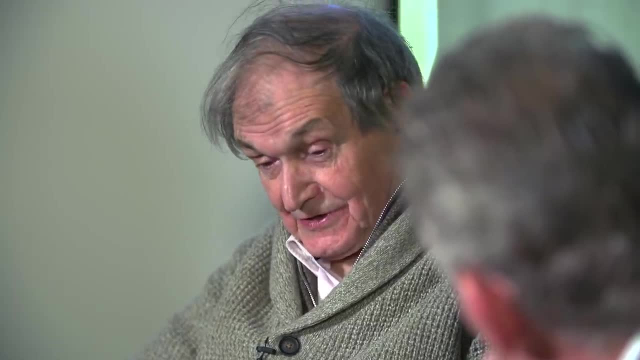 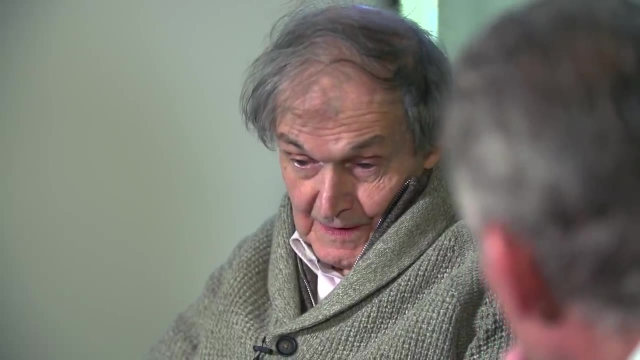 you do with it, according to me, is to say: okay, it tells you that this system has a lifetime And it will, in that lifetime, become one or the other. Without a measurement, It's sort of: that's right. Yes, Without a. 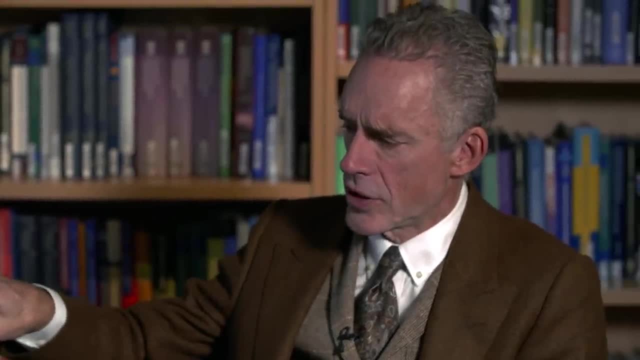 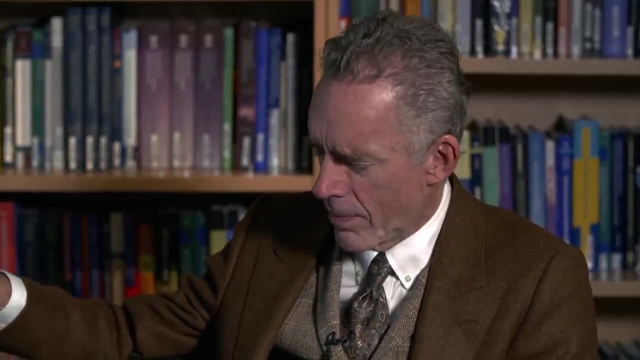 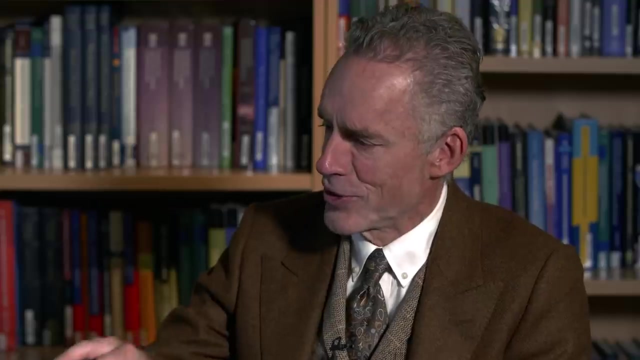 Well, it's so interesting to me that you're interested in consciousness And you see that consciousness in this Goodell theorem sort of manner And I would think I think the most predictable thing for you to believe as a consequence of that would be that it is conscious measurement that collapses: the quantum indeterminacy, the waveform And 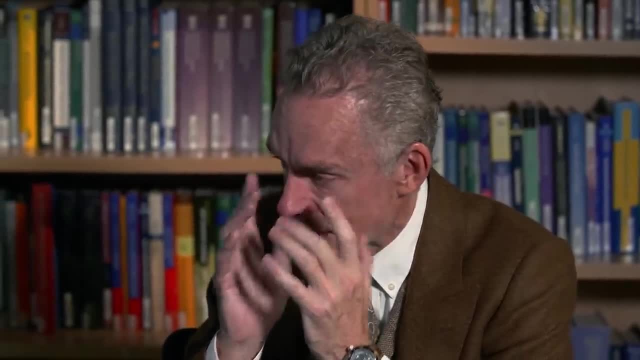 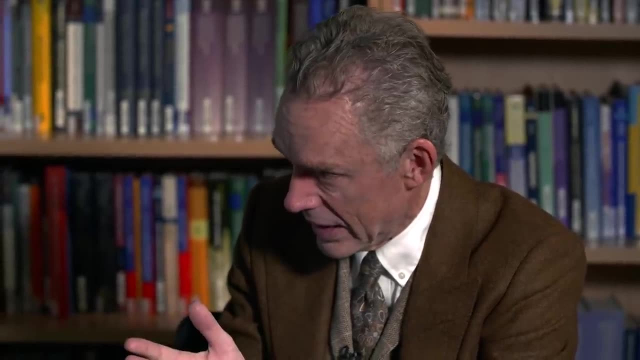 yet you don't. You think that that statistical vagueness will collapse into something that's essentially: Is it either or Is it binary? Is it zero one? the collapse? No, You mean No, there's a probability it'll do one or the other. 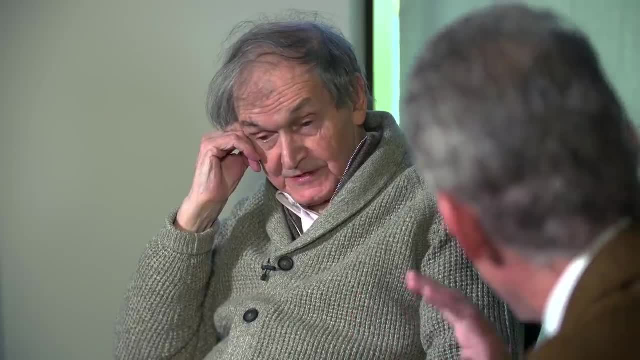